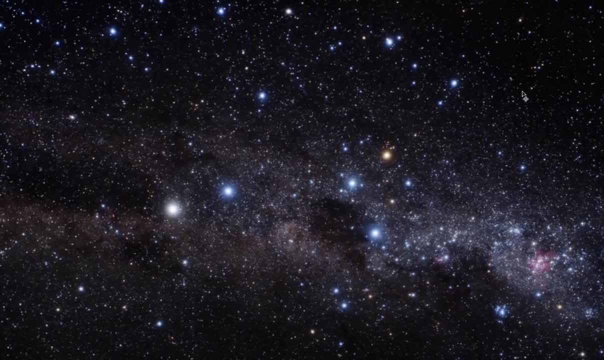 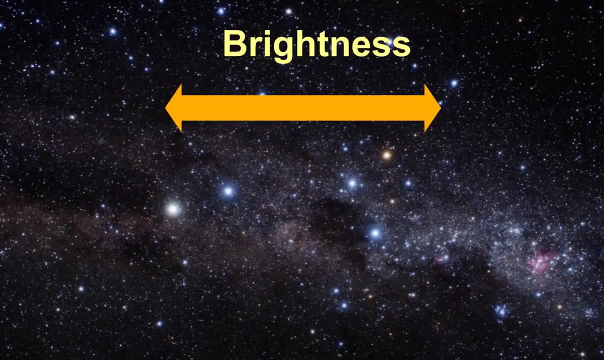 understand the HR diagram, That is, brightness of a star and the color of a star and the information that we understand from those two things. So let's concentrate on brightness. There's two aspects of brightness and the first thing is how bright it just appears And brightness initially. 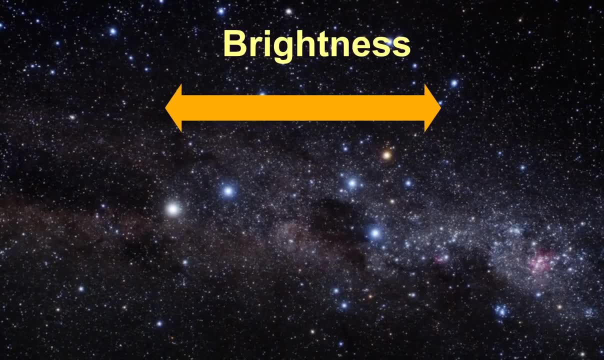 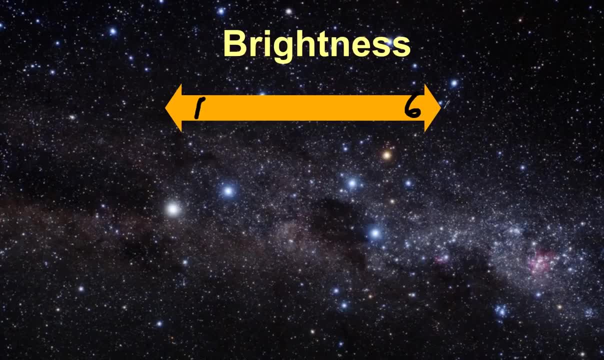 was the dimnest star saw, and anything beyond that, of course, he wasn't able to see. And as far as this was concerned, there is nothing beyond the one, And so we had various categories along the way of brightness, Our modern technology, of course. 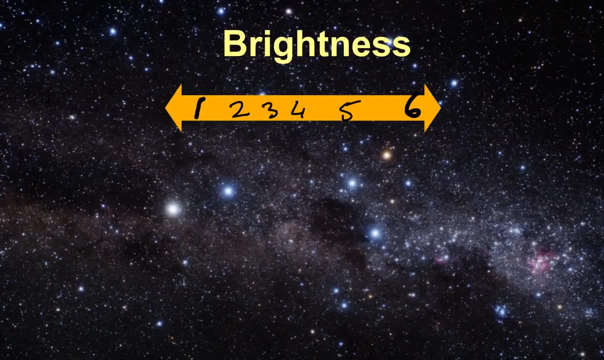 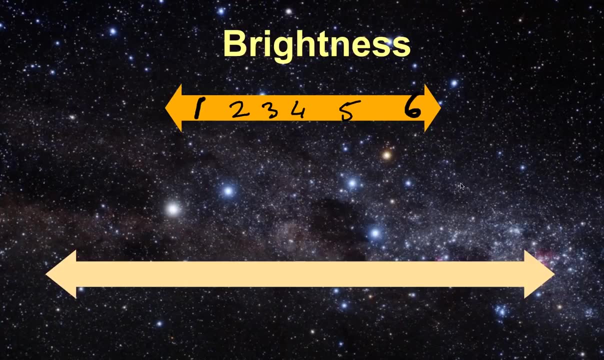 allows us to see however we like us to see further. we are now able to go beyond that so we can get brightness of stars that are beyond six, because now we have telescopes to see dimmer stars. so, for example, this image here: you can clearly see far more stars in this image than you would naturally, even in the best situation. 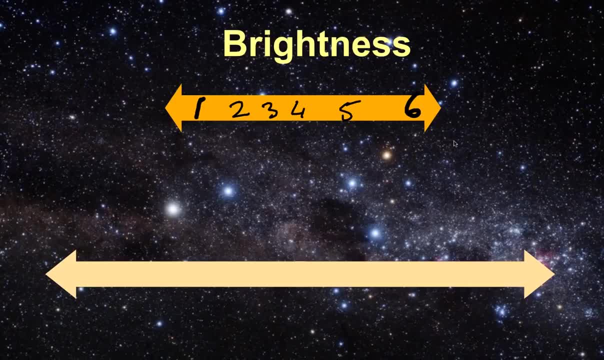 such as out deep in the country without light pollution. if you were to look at the southern cross and saw the pointer stars- as i said, alpha centauri and beta centauri- you would not see all this data because, simply, our eyes aren't able to see that such low sensitivity and clearly we can. 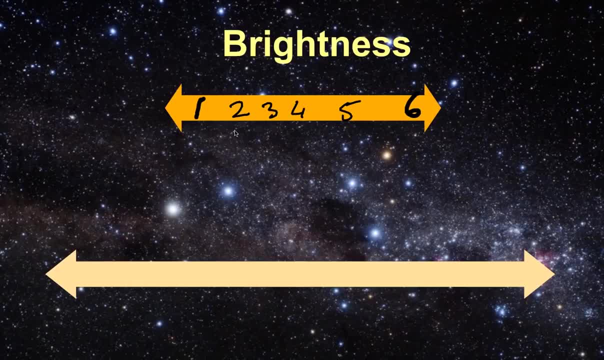 go beyond this too. so, for example, as hipparchus looked at the northern hemisphere, there are stars brighter than his own. so we have numbers that go beyond that, and so we can even have stars that have a brightness of a value that is brighter than one, so even into the negative values. but 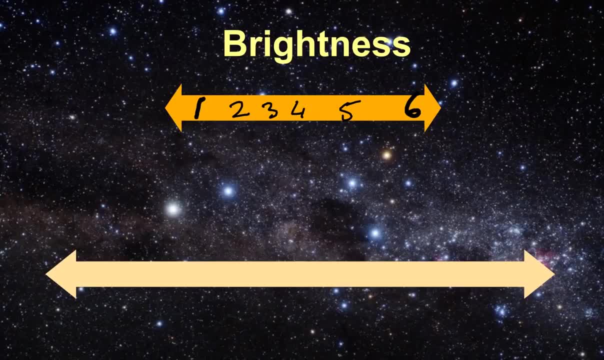 before we go on, we need to also discuss a different terminology here, and so what hipparchus is now referring to is the idea of a star that is brighter than a star. that is brighter than a star in terms of its scale of brightness is a term that we know as apparent magnitude, in other words, 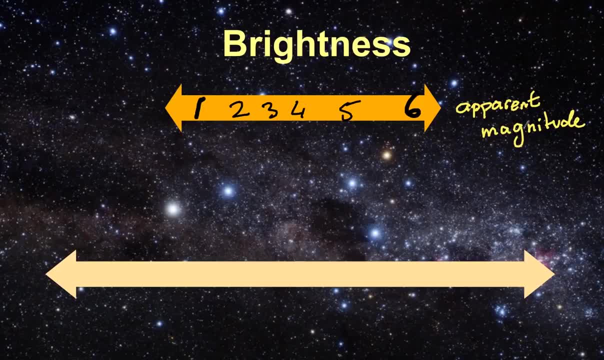 how bright does it appear? what is the magnitude in terms of appearance? now, this scale is now slightly adjusted based on the five jumps over here is equal to a hundred times brightness. so, for example, star that is classified as a magnitude of one is a hundred times brighter than a magnitude. 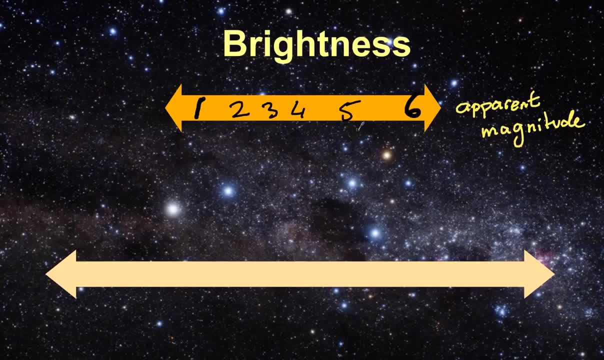 of six, but that will be a discussion of another video in terms of the details. but the other real big issue to understand is that this is how bright something appears and in other words, if we look at, for example, these two stars, they appear roughly equally bright. now alpha centauri has an apparent brightness of 0.01 and beta centauri has an 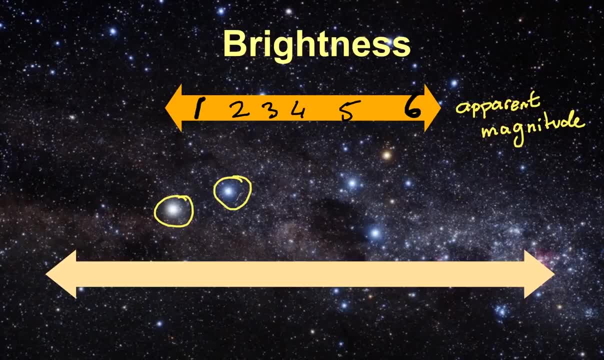 apparent brightness or apparent magnitude of 0.61, which means it's slightly dimmer. but the problem is is that what it doesn't take into account is that it doesn't take into account. the fact that it doesn't take into account is the distances of these stars. now, if i were to take a candle, 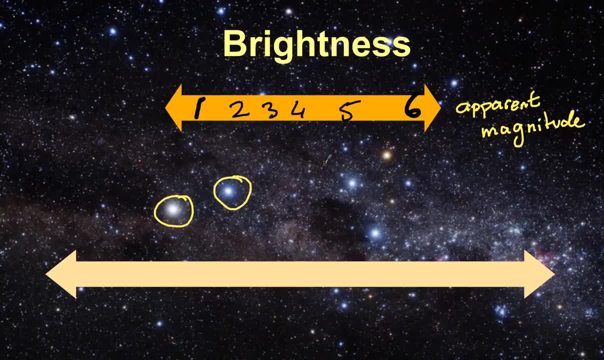 and hold it up, like within 10 centimeters of your eye, then that candle will appear much brighter than, let's say, a floodlight that is 100 meters away, even though the candle is inherently less bright than the floodlight, and so we need to adjust this apparent magnitude to account for. 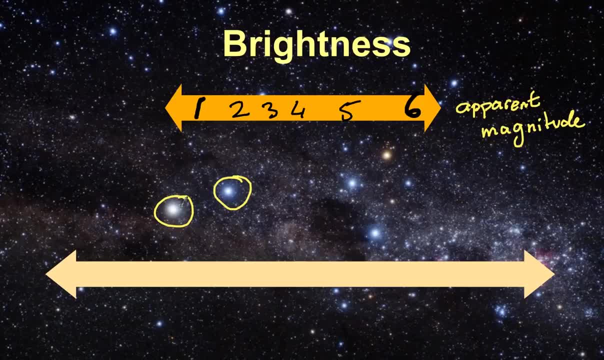 the distance now to give you a perspective, alpha centauri is 4.3 light years. okay, so in fact, this system here is the closest star system apart from our sun. beta centauri, even though it appears approximately the same brightness, is 390 light years away, so significantly further. so clearly. 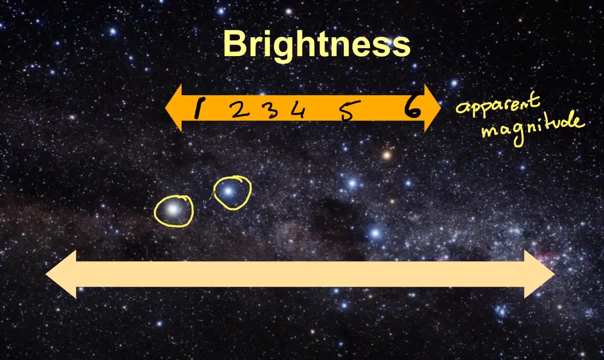 star must be significantly brighter than this one, but of course the distance screws the situation up for us, so we need to adjust that, and in order to do that, we need to know the distance. now i won't go into the specific details of how we determine stellar distances, and in fact there 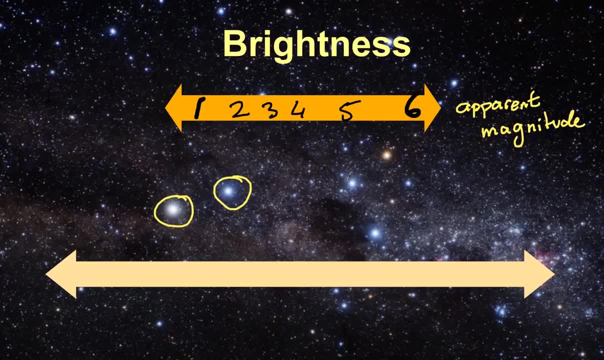 are two methods. for stars that are roughly around 300 light years away and less, we have a system called stellar parallax. and any stars that are significantly further away, we use a way of working at distances by referring to cepheid variables, but that is a topic of another video and you're 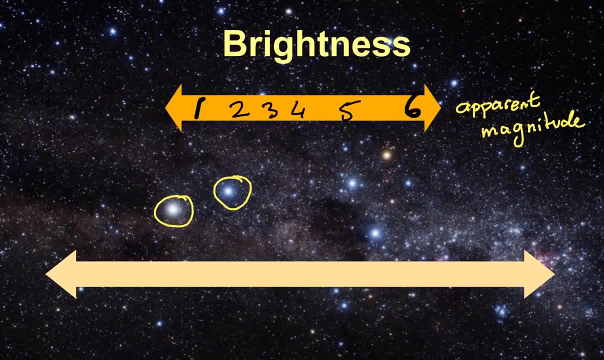 free to look that up and i will probably organize to do another video based on how we determine stellar distances. but, needless to say, we have ways of determining distances and therefore we have a way of adjusting the stellar distances, and we can do that by using a method called the 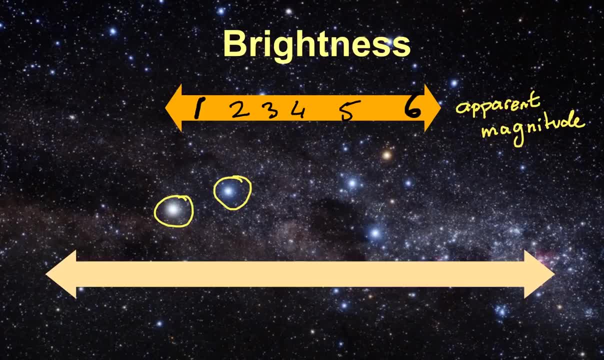 star's brightness to what we call its true brightness or its true magnitude, and we call that the absolute magnitude. so, for example, as i told you, alpha centauri has an apparent brightness of 0.01 and i told you that beta centauri has an apparent brightness of 0.61. 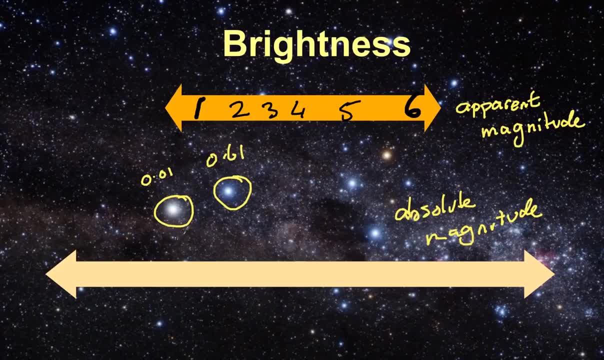 and so clearly they look equally bright. but because this is further away, we can now adjust that. so we get 4.38 for the absolute magnitude for alpha centauri, but negative 4.53 for this one. so this is significantly brighter in reality. so this actually reflects the star's true brightness. 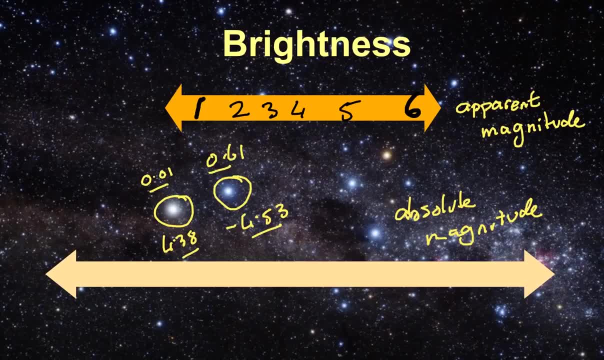 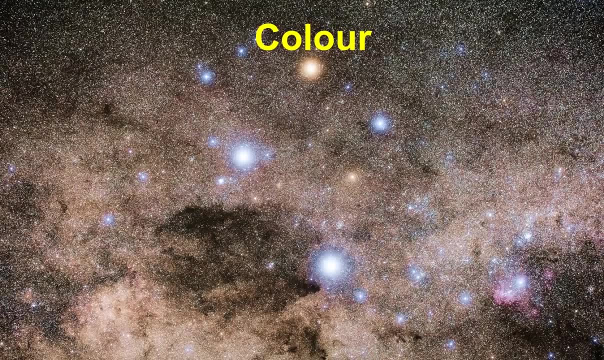 as opposed to what it appears. so that's brightness for you. now, we can classify stars according to their brightness. however, here is again a southern cross, and even in this case, you can even see more resolution and more stars. secondly, though, we need to look at color, and it is clear that this star is a different. 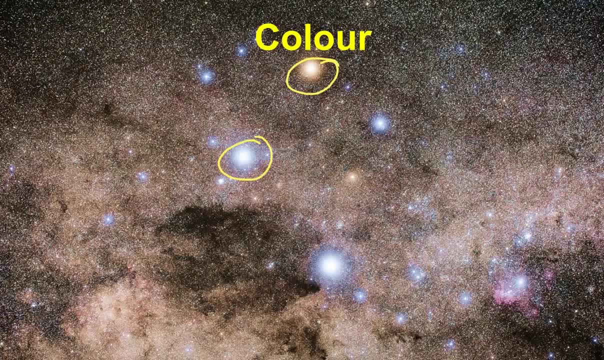 color to, let's say, this star, and why is it different color? well, color actually gives us an indication of a star's temperature. now i have a video already where i discuss stellar classification and also one that discusses winslaw, but we have a way of understanding the temperature. 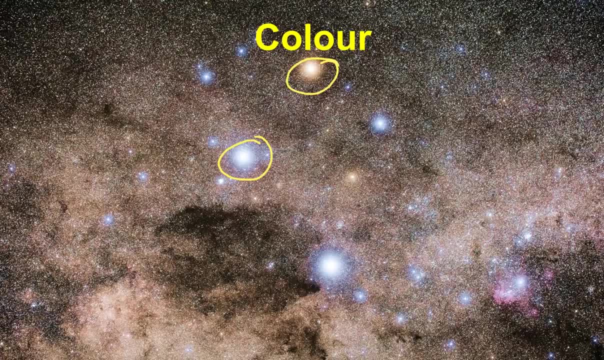 of a star by examining the color of the star, and so once we have an understanding of the color of the star, we can determine its temperature and, as a result, we know that stars can have a varying temperature of anywhere between 3000 kelvin up to 50 000 kelvin. now we are talking about, of course, 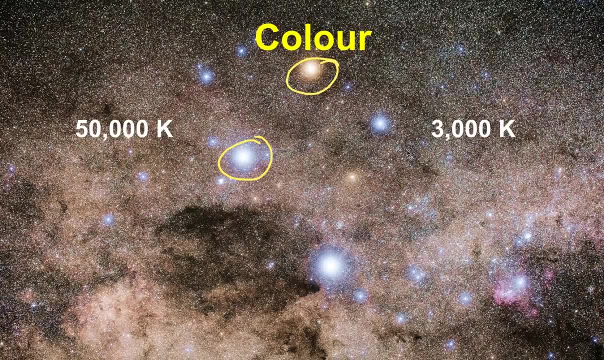 the surface temperature of the star. internally it's into millions of degrees kelvin. we now have a range. we can now classify stars according to the color, in terms of the cooler stars and to hotter stars, and the cooler stars will appear redder and the hotter stars will play bluer. we can 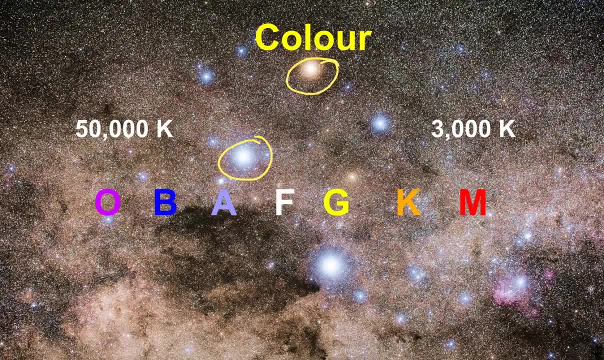 then also have a different way of classification. we have a system which is a letter classification. we give a star, a classification of anything from a, o down to m and b, a, f, g, k and m, and in between we can have an o1 or an o9 and the range and so forth. we can have an f2 star and so forth. 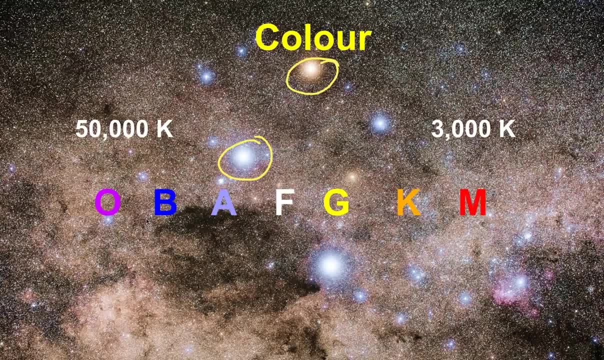 and one quick way to remember these letters, if you want to, is to remember a mnemonic that's quite old and a little bit sexist, but it's one that's stuck around basically for almost a century and it's basically: oh, be a fine girl or guy and 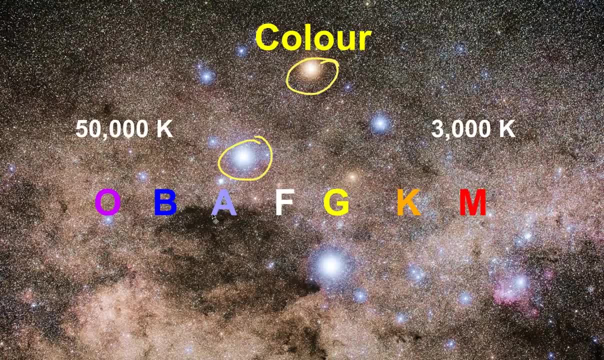 kiss me. so that's a way of memorizing the classification system of stars according to the color or according to their temperature. so now we have two things: we have brightness that we classify a star with, and its color or its temperature. so now let's start looking at a graph. so here i have a graph and 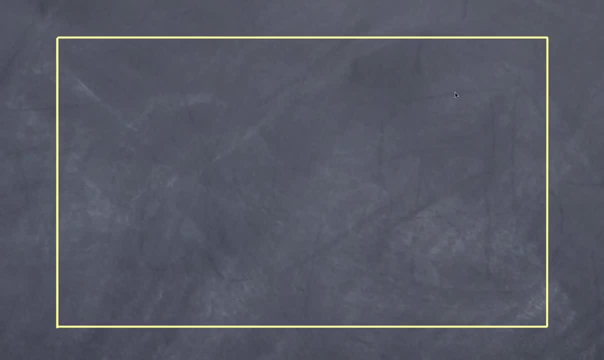 like a normal graph. we're going to actually have two sets of y-axis and two sets of x-axis. the first thing we have here is magnitude, and that is specifically the absolute magnitude. so stars, true brightness, and, as you can see, we start with really dim stars down the bottom to really 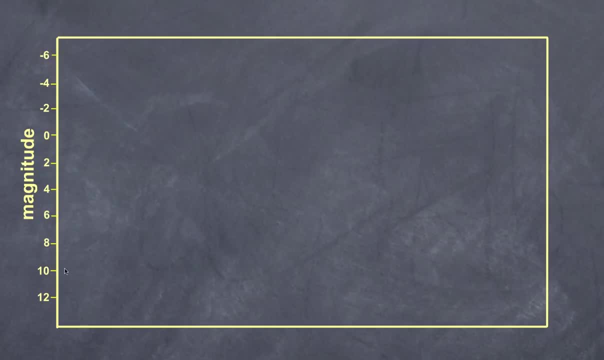 bright stars up the top, because the order of the magnitude is that the bigger the number is, the brighter the number is. we're following hipparchus's initial classification system. now we could also do that in terms of luminosity. now, luminosity is the amount of energy star releases, and it's 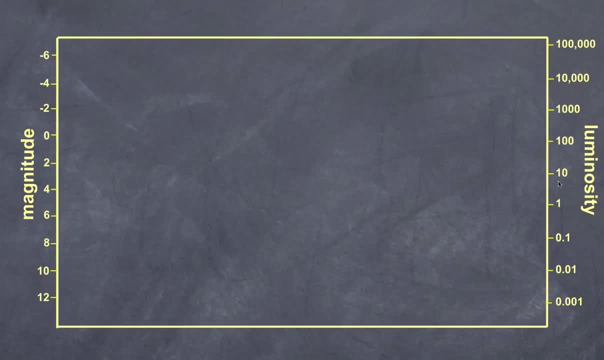 obviously related to brightness, though there is a slight mathematical difference between the two, but nonetheless we can classify stars. so our star, our sun, is approximately 4.3 in terms of magnitude, and so what this does is this number, rep one represents the number of luminous stars that we have in our solar system, and so we can see that the number of 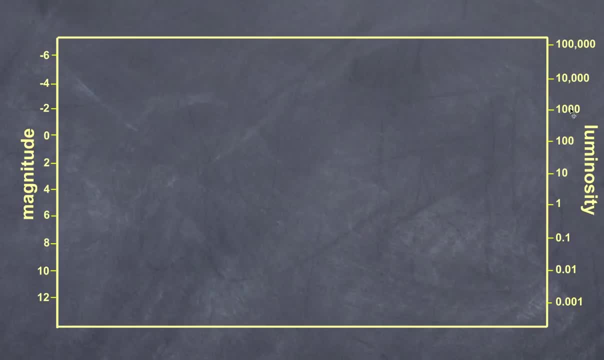 luminous stars that we have in our solar system is more luminous compared to our sun, and so as we go up, you can see we have- we classify- stars that are 10 times more luminous than our sun, 100 times one thousand, ten thousand, hundred thousand and so forth. down here what you should automatically see. 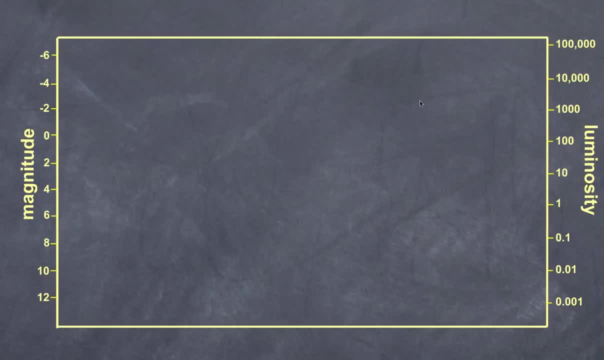 that this scale is not a linear scale. it's a lot we call a logarithmic scale, and so, rather than going up in additions, we're actually going up in multiplication. so it's a logarithmic scale, so we're actually going up in multiplication. so we're actually going up in multiplication here. 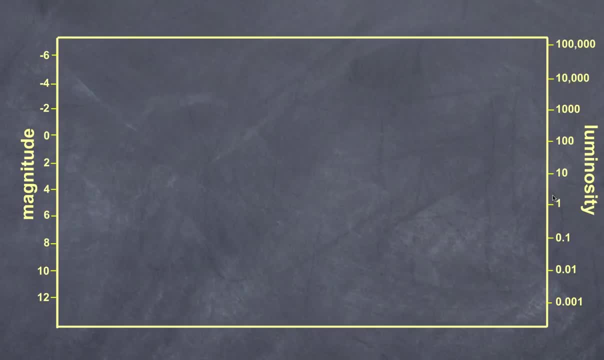 and so we're actually going up in multiplication here, but it's more similar to the linear scale. so if i look at the right of our star, we should see that it's significantly brighter than our sun, or significantly luminous in our sun. that takes care of the y-axis. what about the x-axis? well, Down here we of course have the stars according to their classification, from o to m, and up the top we have a similar scale that tells us the temperature, and again, you'll notice, is that it's not a pure linear scale. we have, down this end, hotter stars, and down in this end, we have more hot stars, and down this end we have more heat. 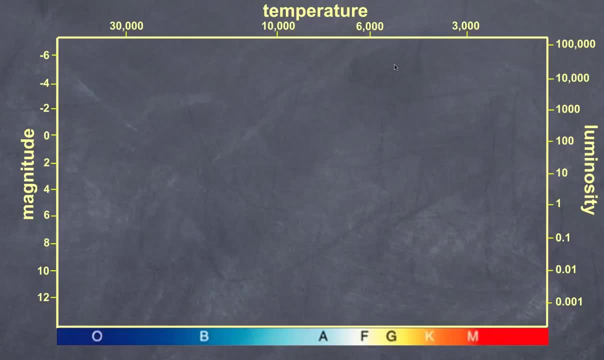 we have cooler stars and up the top, of course, we have brighter stars, and then the bottom we have here, if we go via the y-axis, we have dimmer stars And clearly, of course, if a star is hotter, 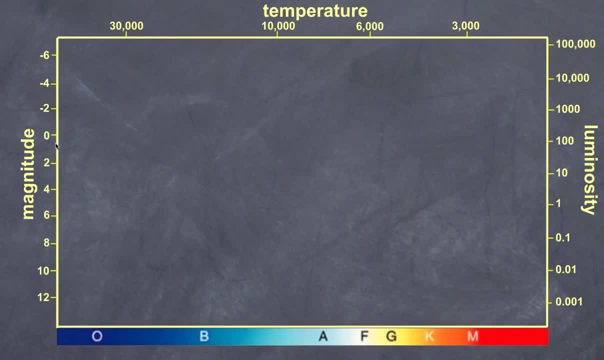 it's going to be generally brighter as well, but, as we'll discuss in a moment, there are other variables that determine the brightness as well. So what happens if we start to plot stars according to this scale? So what do you see? In this case, I've plotted various points to represent stars. 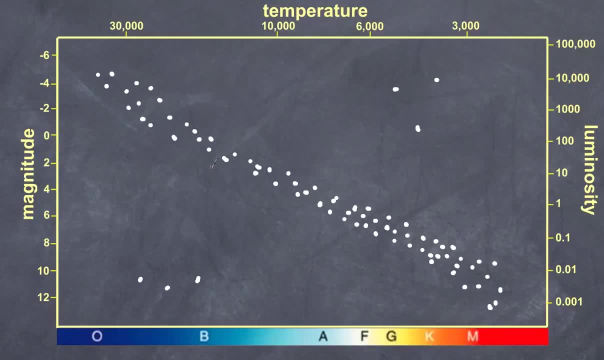 that we have classified in our local area of our galaxy, and this is not particularly accurate, obviously, but it does represent what we do get in terms of stars, and the first thing you'll notice is that the stars are not as bright as they used to be. So what do you see? So what do you see? 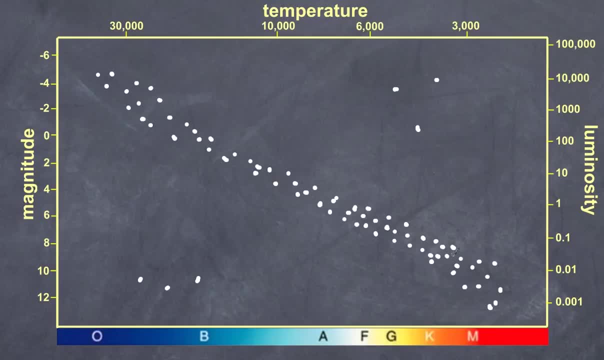 The majority of the stars seem to fit on this line. In fact, 95% of all stars fit on this particular line. We call this the main sequence, this almost classic S shape of stars. So what does that actually tell us? Well, so over here we have stars that are not very bright and they're also not very. 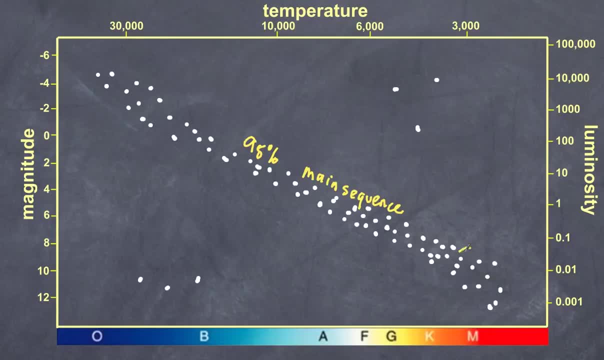 hot. So clearly they're also quite small. They're not big stars. If we go up to the top of the main sequence, these stars, well, they're very bright, clearly, but secondly, they are also very hot. 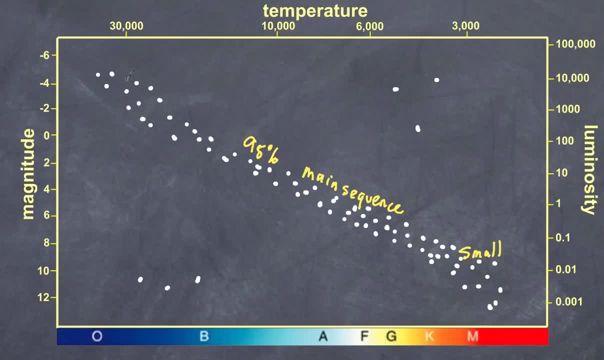 and, as a result, because they're bright and also they're very hot, we know that these stars generally are large. The other thing, of course, too, to remember is that these stars being hot and very bright, they are under a very high temperature. So we know that these stars are. 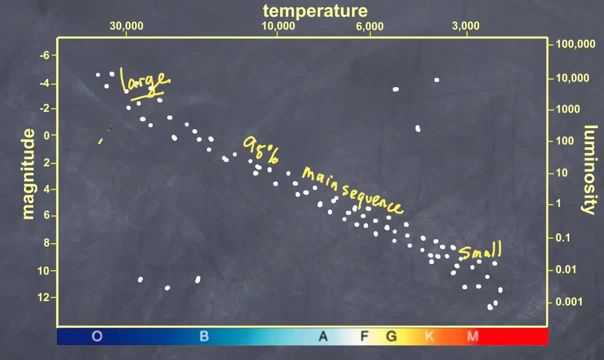 going fusion at a really great rate, And so, generally speaking, their lifespan is measured in 10 to the power of seven years, So they don't last that long, which also explains why we find fewer stars up in this range than we do down here, If we go down the scale these stars have. 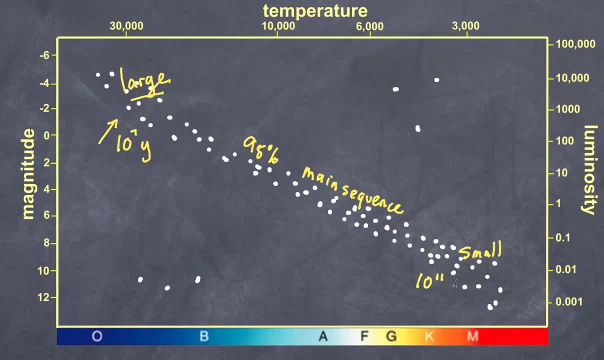 anywhere up to 10, to the power of 11 lifespans, So we're talking about 100 billion years here they could survive. So it's clear that being smaller and obviously going through fusion at a lower rate because it's not as hot- these have a longer lifespan. 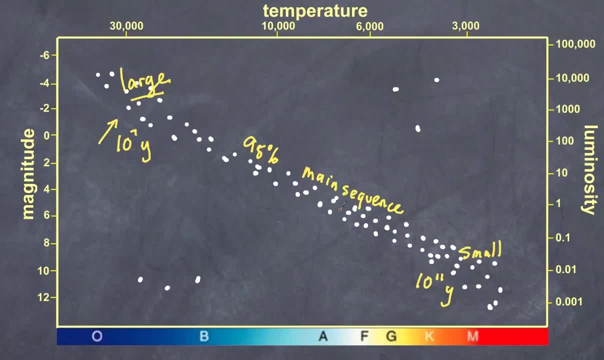 Now our sun sits approximately here in the scale, So it's a G class star, It's a G2 star, in fact, And of course its luminosity is equal to one when compared to our sun. So that's the main sequence. But then we have these stars over here and these few stars over. 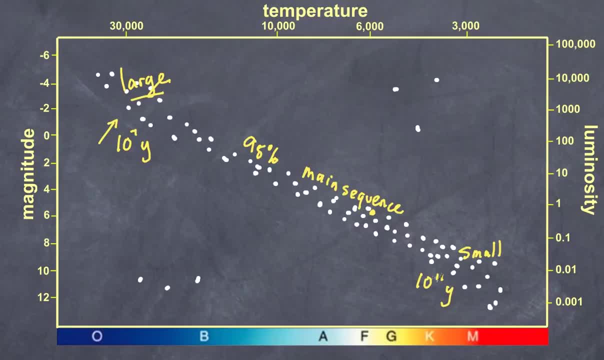 here. What do they represent? These guys are clearly not hot stars. They're cool stars, But they are very bright still. In fact, their brightness is equivalent to some of these blue stars over here, So they're still very bright. What would 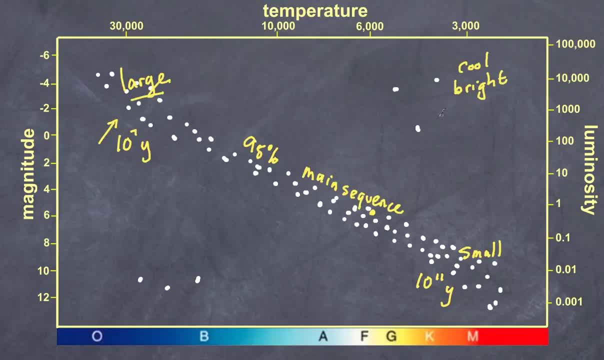 contribute to the fact that they're cool but also very bright. Well, obviously, what that means is that they are very large. So these are we often would call the giants. Now, in fact, you can go further into that. We have actually 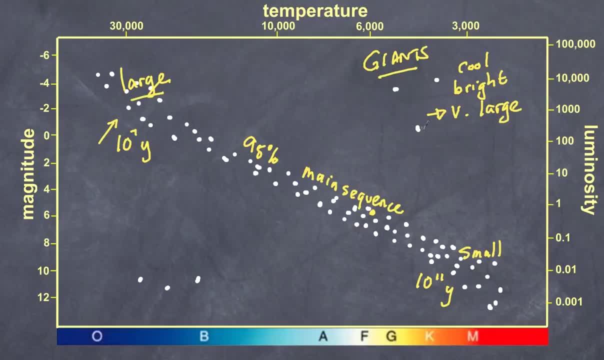 these ones here which are called the supergiants, And then we have here who are the giants? Over here we have stars as well, But in this case the star is extremely hot, but it's not very bright. So it's very hot but not bright. Why is that? Well, 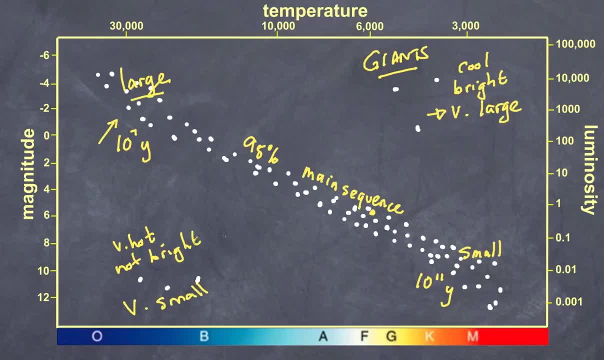 they must be very small. So these stars are what we refer to as white dwarfs, And white dwarfs, they're extremely small. Now let's give ourselves a bit of perspective to help us understand that. So what about these large stars over here? Well, here is an example. 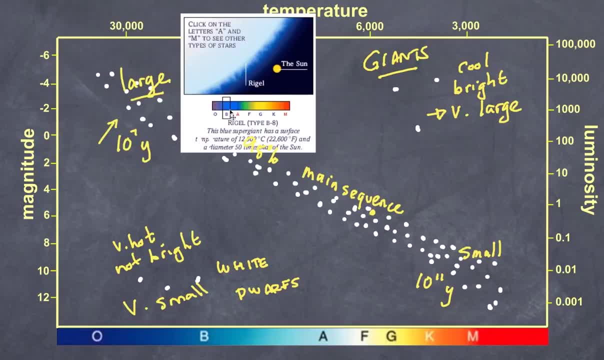 of the large star, And so Rigel is a blue giant. It's a B-class star, B8, in fact, It's very hot. Its surface temperature in terms of Celsius is 12,500 degrees. That's in this range, And you can see that, compared to the Sun, it is large. What about the giants over here? 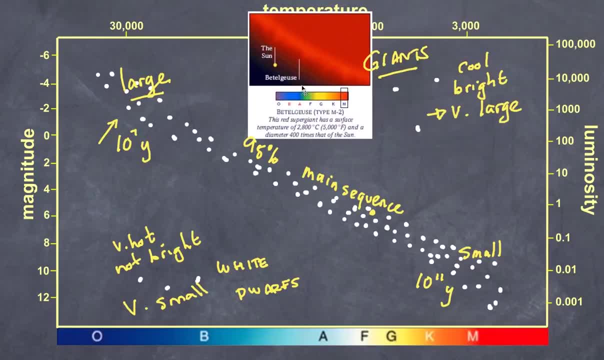 And again, if we look at the giants, a good example is Betagoose, And Betagoose can be found in the constellation of Orion, And it is extremely large. Now it's an M-class star, an M2.. So it's. 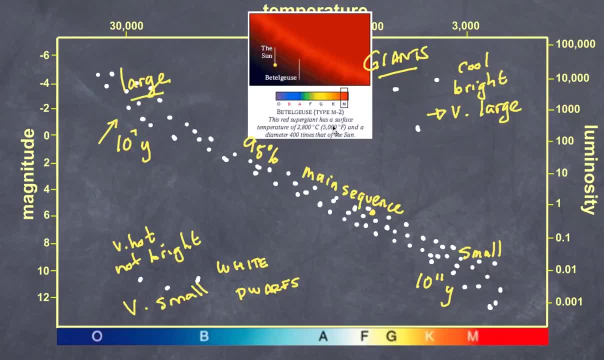 not very hot- 2,800 degrees Celsius or 5,000 degrees Fahrenheit for the American listeners- And its diameter is about 400 times that of the Sun. Now, it is very significantly large. If we were to replace the Sun with Betagoose, then Betagoose would consume. 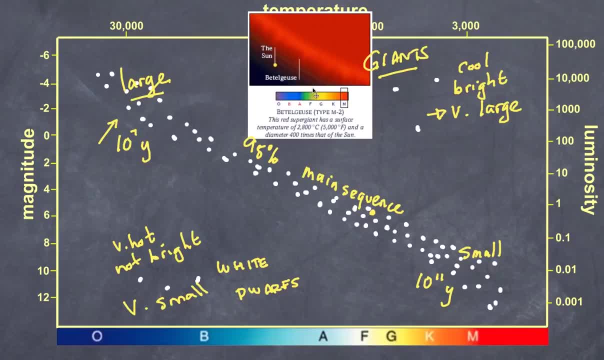 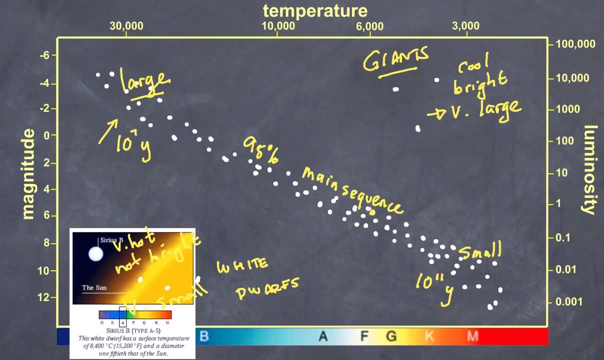 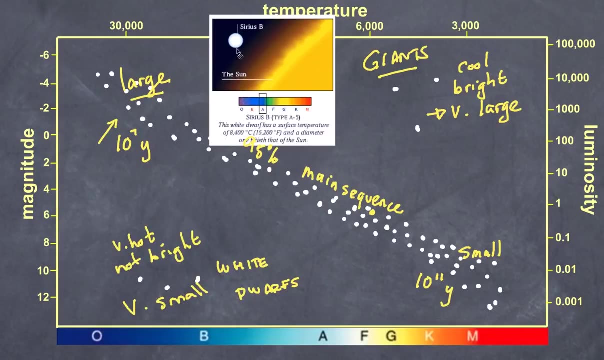 not only the inner planets, but stretch as far as Jupiter. So we're looking at a really massive star here, But then there, on the other end of the spectrum, we have these guys, And this is an example of Sirius B. It's a white dwarf, It's hot, but clearly it is very small. And how do we know? 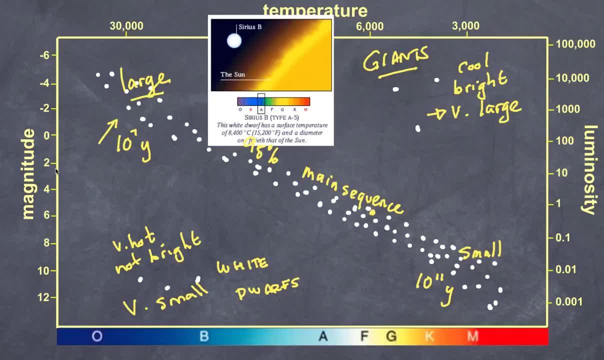 all this Simply because we can determine it mathematically by examining the star's magnitude and the star's magnitude, And we can determine the magnitude of the star's magnitude by examining the star's magnitude and the star's magnitude, And we can determine the magnitude of the star's. 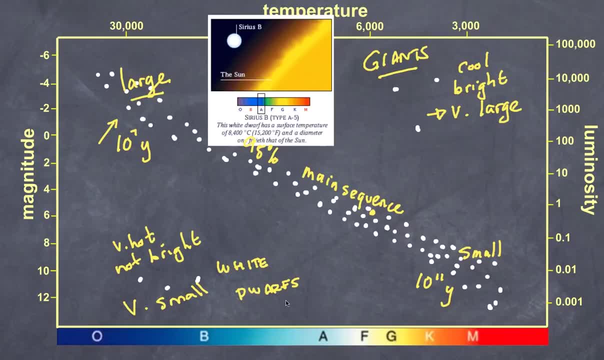 color or temperature and therefore work out the star's size. So that is the HR diagram. The HR diagram, as I said, Y-axis, deals with brightness, with brightness up further high and dimmer further down. and temperature, with the hottest at the left hand of the scale and coolest. 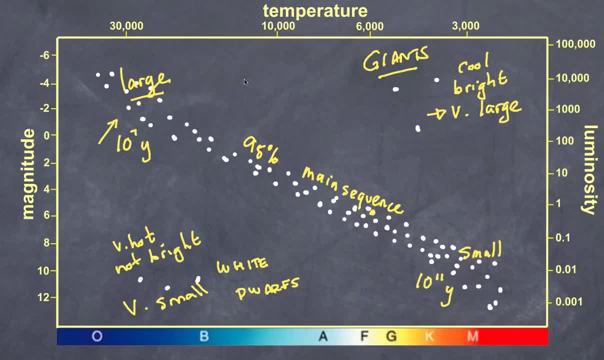 in the right hand of the scale. If you plot all the stars that we have in our local area that we can measure, we can measure the temperature of the stars And we can measure the temperature of the stars at the start of the solar辯젤 calendar, We find that 95% will sit onto this area called the 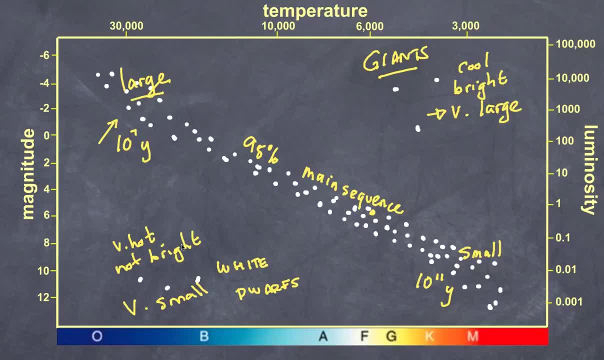 main sequence, with a few sitting in the giant's phase and a few sitting into the white dwarf phase over here. I hope that's helped you understand the worldませq entonces, I fuck that up to 35% in the worldI hope that's helped you understand the HR diagram. Thanks for watching. Bye for now.